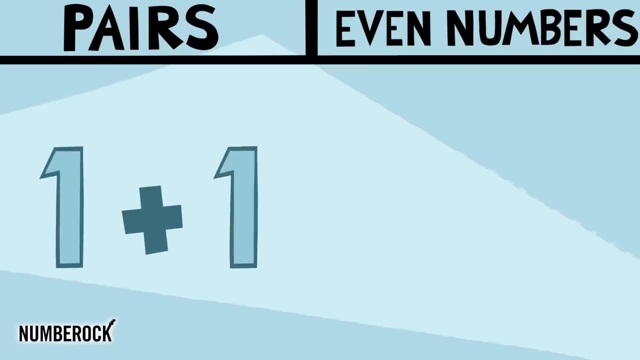 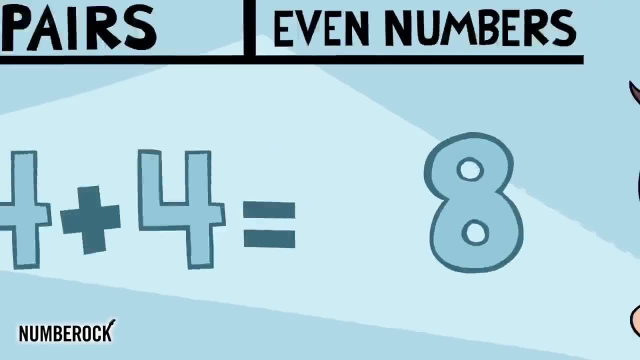 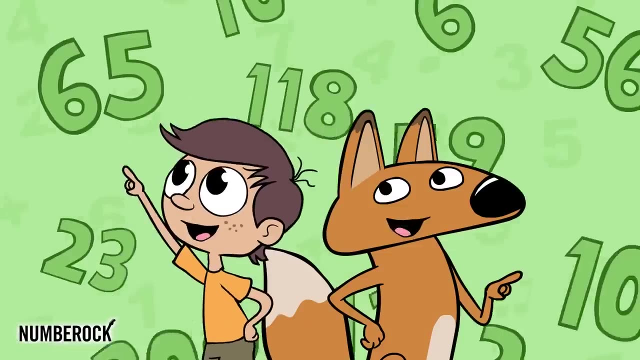 down the middle. If they make pairs, you solve the riddle, Because one plus one equals two and two plus two makes four, It's true. Then three plus three equals six and four plus four makes eight. big sticks Numbers big and small. Today we're gonna count them all. 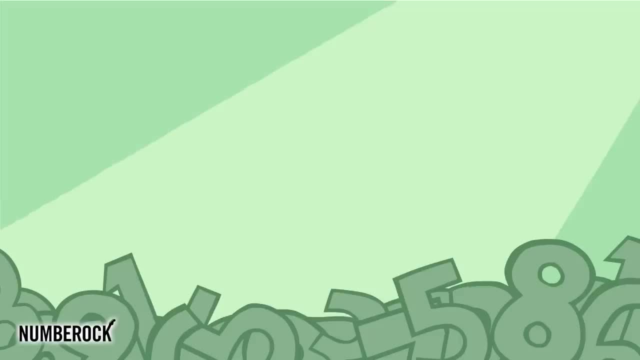 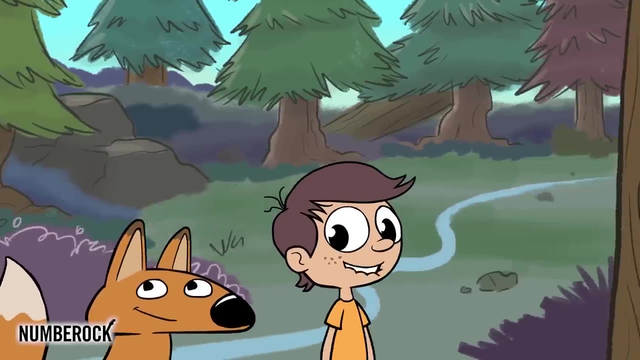 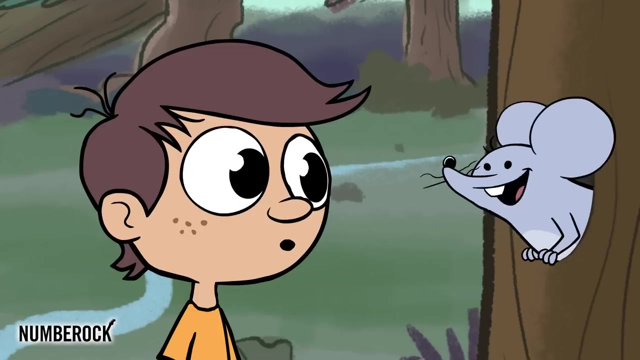 Some are even some are odd. Won't you join our counting squad? We walked further into the forest when a rat squeaked. Please sit with me and be my guest And I'll take the time to show you how to tell which numbers are odd. We looked at the fox and 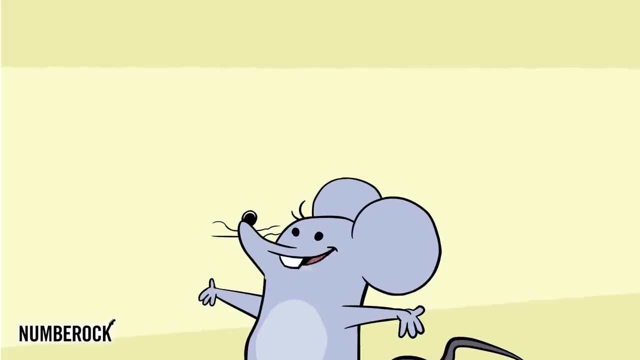 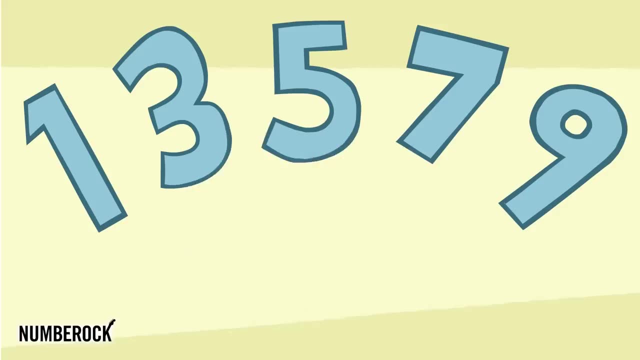 she gave a sly nod. The first five odd numbers in line are one, three, five, seven and nine. They are not divisible by two and for all odd numbers, the same is true Between one and ten. there are five of them. Now I'll count the odd numbers. 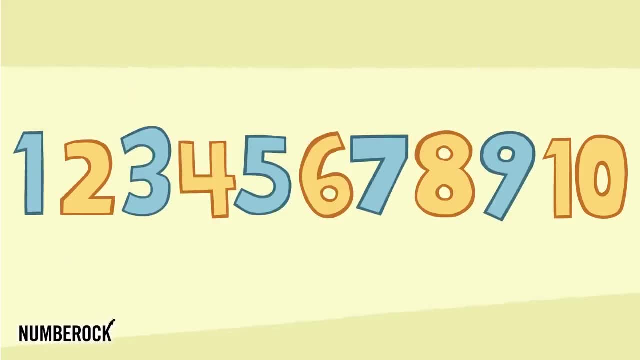 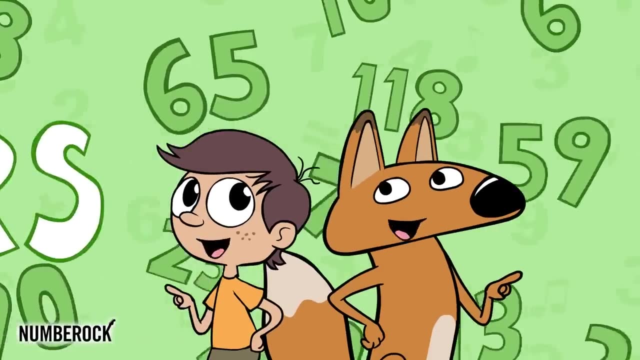 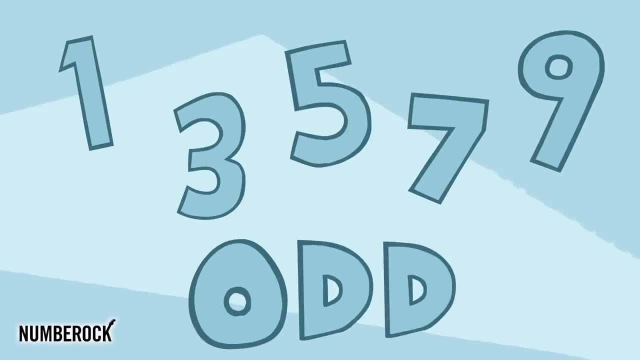 again. One, three, five, seven and nine. They're every other number on the number line, Numbers big and small. Today we're gonna count them all. Some are even, some are odd. Won't you join our counting squad? 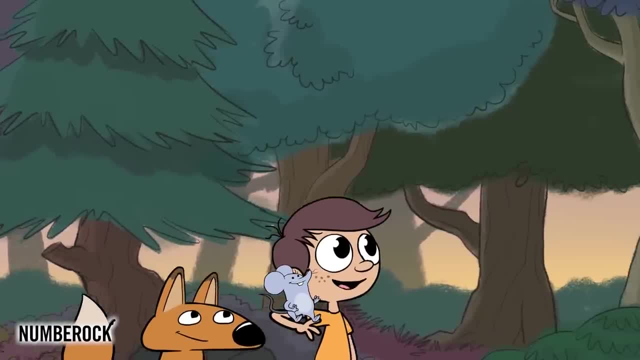 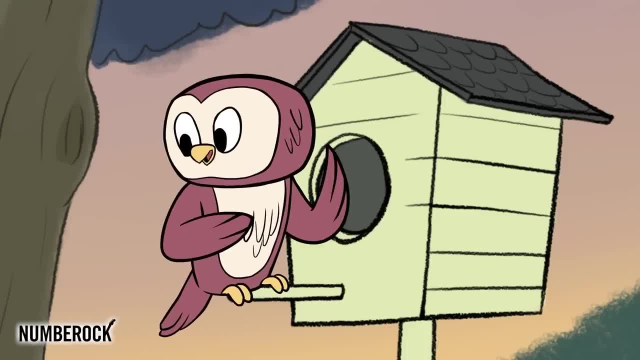 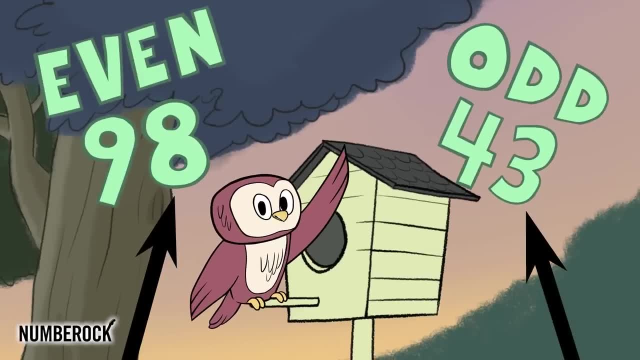 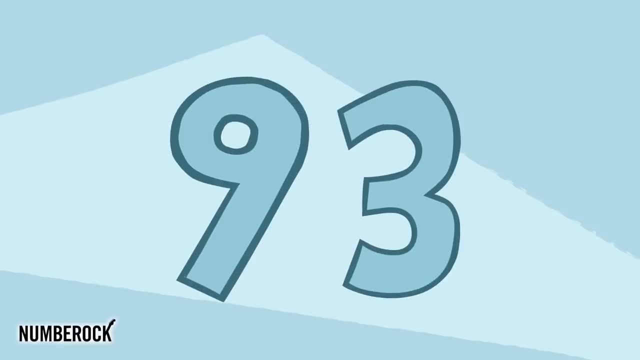 Please visit with me just for a short time and I'll discuss bigger, even and odd numbers, as I rhyme. Bigger numbers are even or odd too, and the last digit holds the clue. So what about the number seventy-two? It's even because it ends in two. Or what about the number ninety-three? That number's. 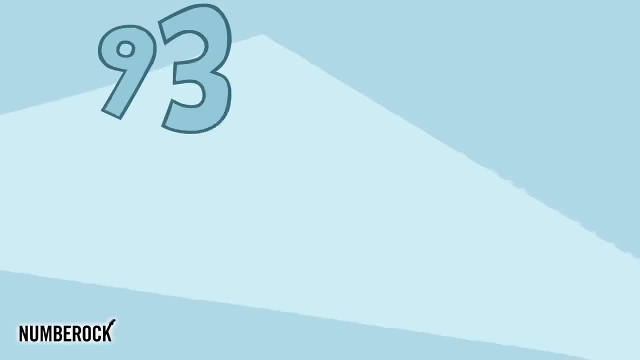 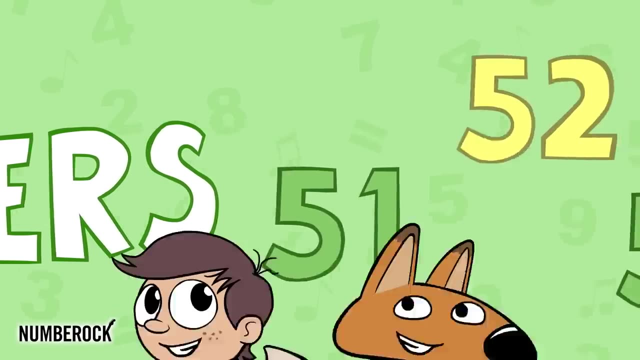 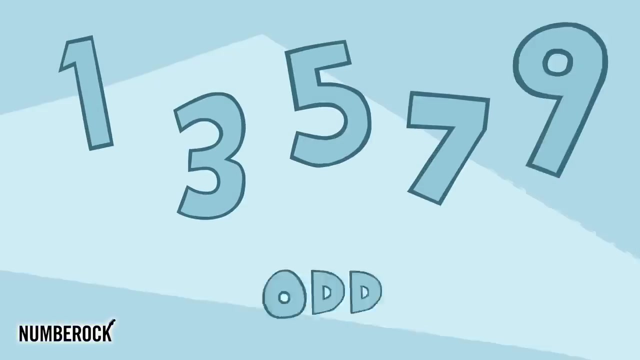 odd because you see the last digit's, the odd number three, which means it can't be split evenly. Numbers big and small. Today we're gonna count them all. Some are even, some are odd. Won't you join our counting squad? 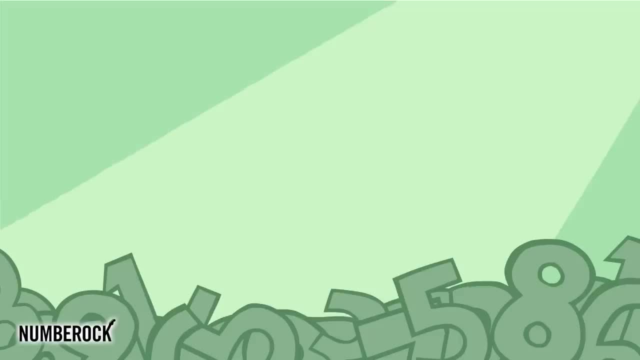 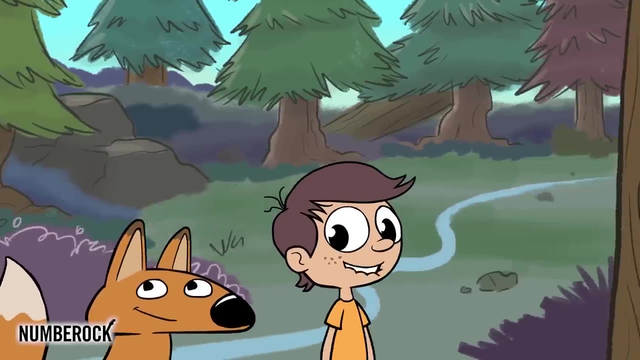 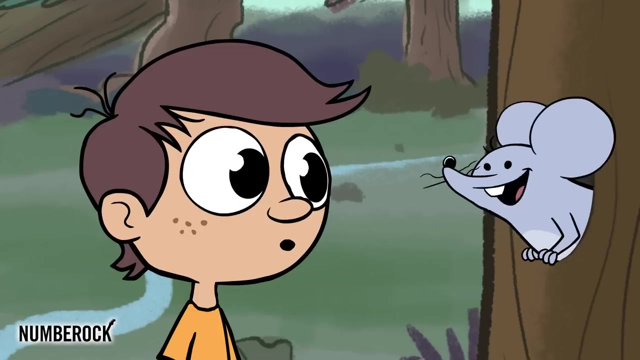 Some are even some are odd. Won't you join our counting squad? We walked further into the forest when a rat squeaked. Please sit with me and be my guest And I'll take the time to show you how to tell which numbers are odd. We looked at the fox and 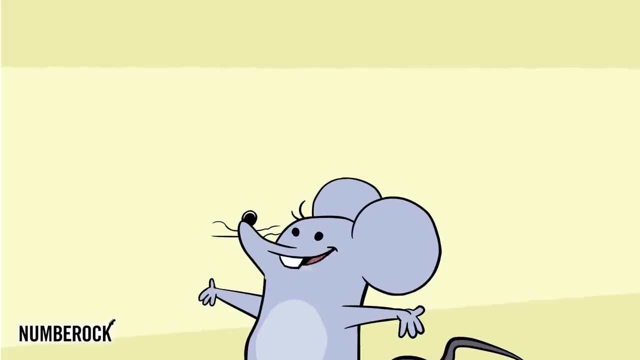 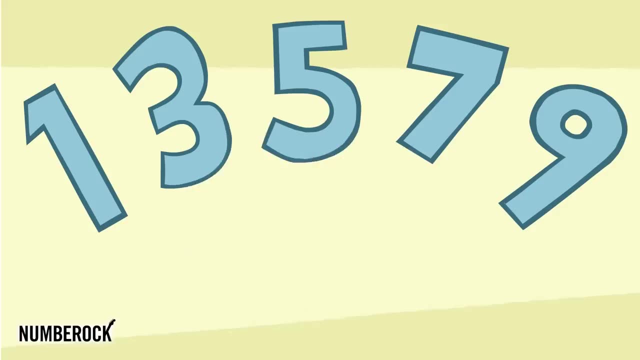 she gave a sly nod. The first five odd numbers in line are one, three, five, seven and nine. They are not divisible by two and for all odd numbers, the same is true Between one and ten. there are five of them. Now I'll count the odd numbers. 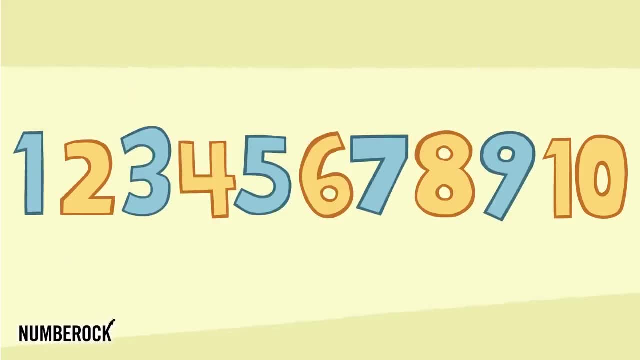 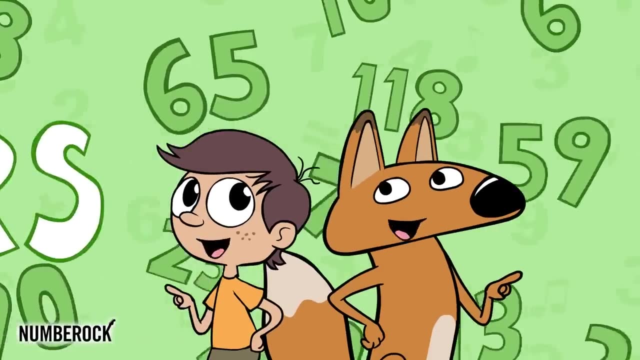 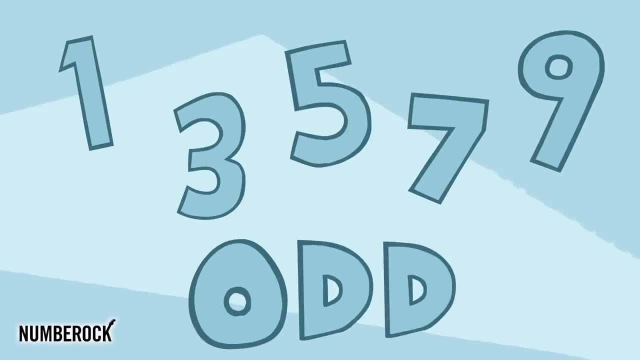 again. One, three, five, seven and nine. They're every other number on the number line, Numbers big and small. Today we're gonna count them all. Some are even, some are odd. Won't you join our counting squad? 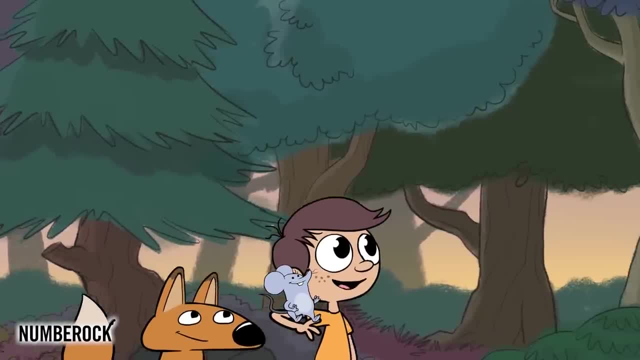 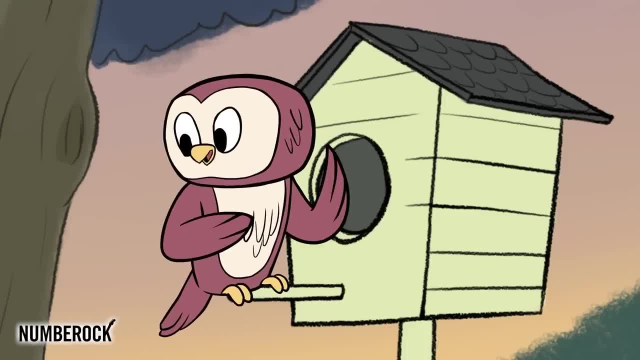 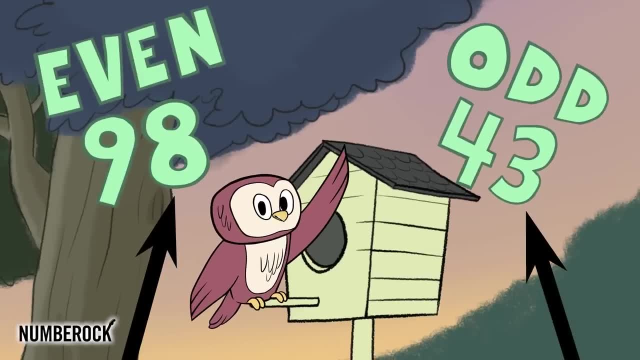 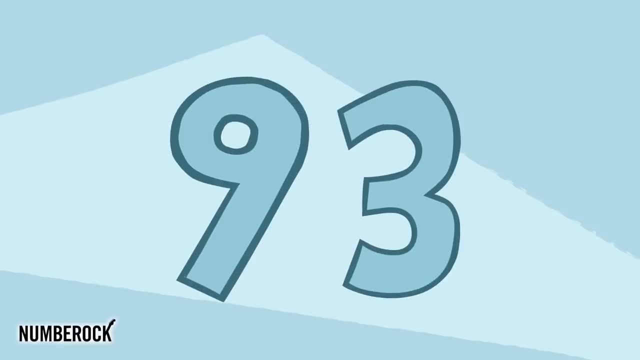 Please visit with me just for a short time and I'll discuss bigger, even and odd numbers, as I rhyme. Bigger numbers are even or odd too, and the last digit holds the clue. So what about the number seventy-two? It's even because it ends in two. Or what about the number ninety-three? That number's. 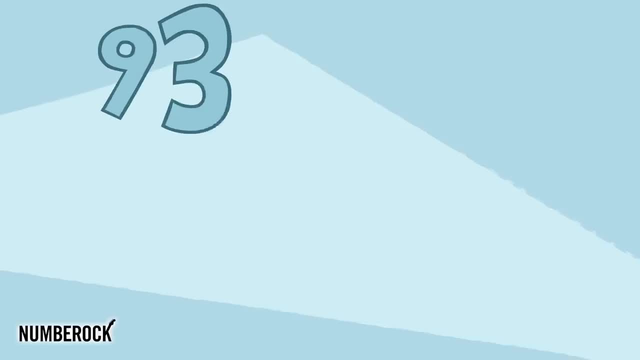 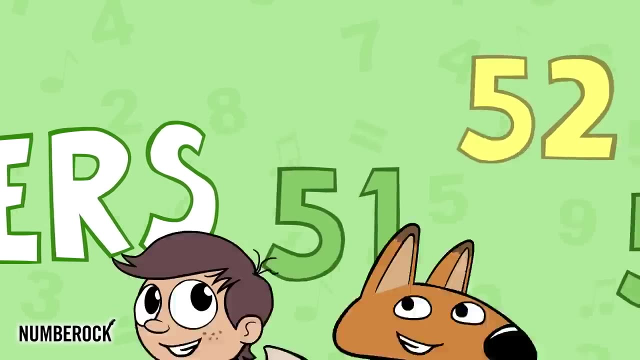 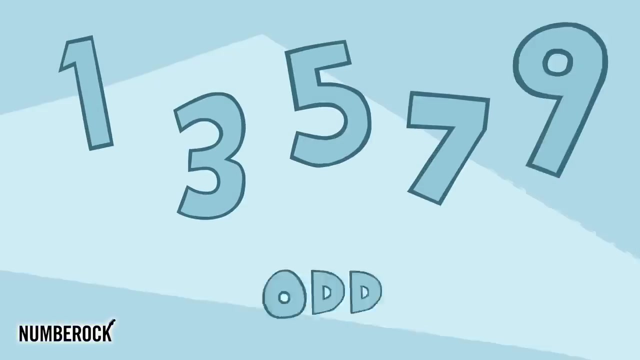 odd because you see the last digit's, the odd number three, which means it can't be split evenly. Numbers big and small. Today we're gonna count them all. Some are even, some are odd. Won't you join our counting squad? 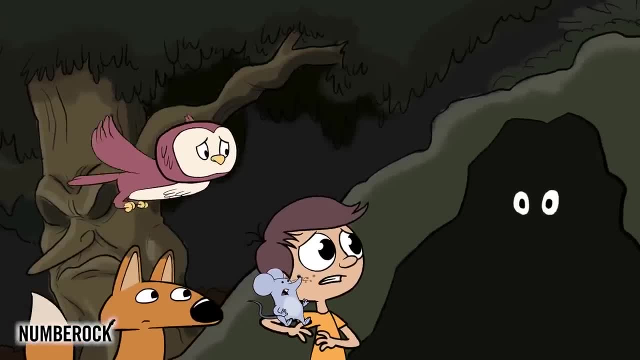 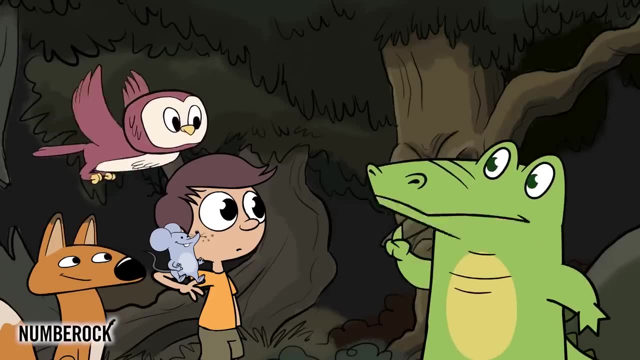 We wandered further into the wilderness, An alligator appeared from the darkness. G'day mates. I've got a special number for you. I've got a special number to teach you, For you must learn about zero before your journey's through.